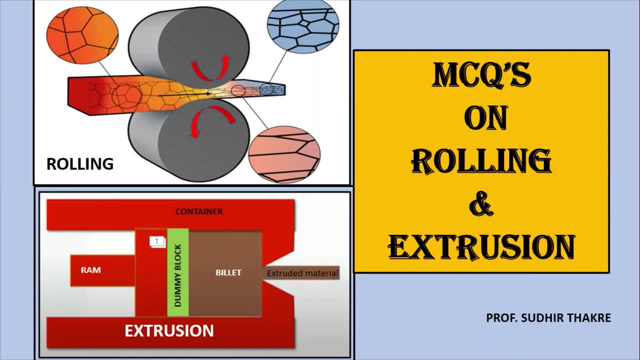 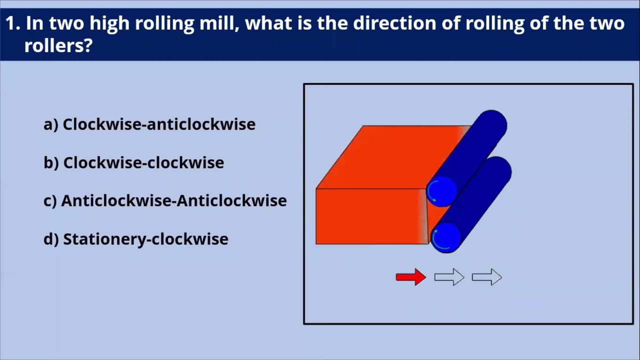 Hello friends, today we will discuss MCQs on rolling and extrusion process. I will explain every answer with the help of appropriate diagram and videos. So let's begin with the first MCQ In too high rolling mill. what is the direction? 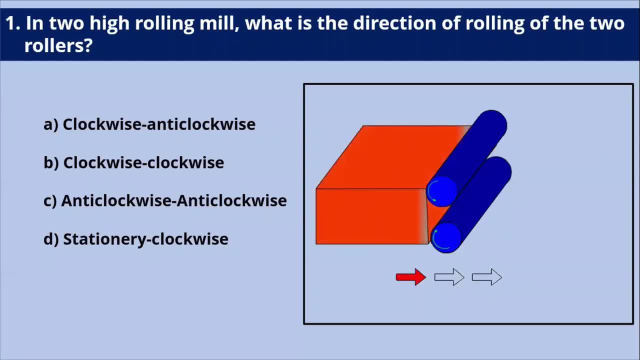 of rolling of the two rollers. In too high rolling mills, the direction of both the rollers is opposite to one and other, Hence one clockwise, while the other will move in an anticlockwise direction, and that's why we can say that in the too high rolling mill the direction 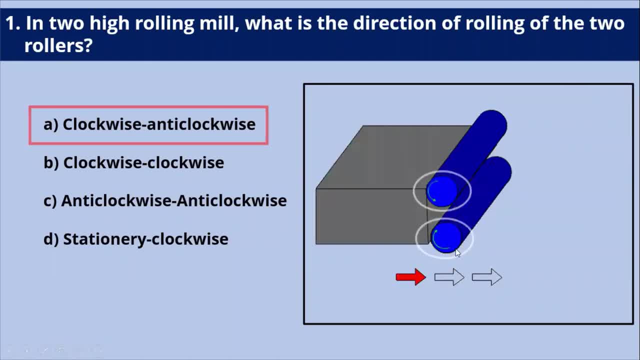 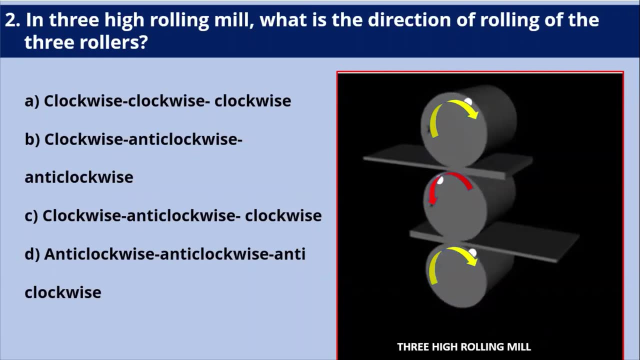 of the rollers are in clockwise and anticlockwise direction, and that's why our answer is A Next question: In three high rolling mill, what is the direction of rolling of the three rollers? So if you see in this diagram, in the three high rolling, 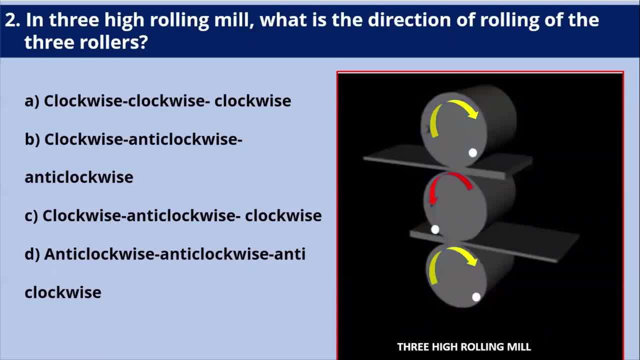 mill. the direction of the roller in the top and bottom are same And the direction of the roller in the middle is opposite to the remaining two, And that's why we can say that our answer is: you can see the clockwise, anticlockwise and the clockwise. 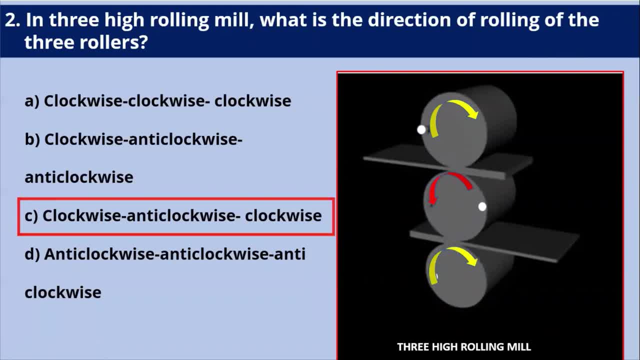 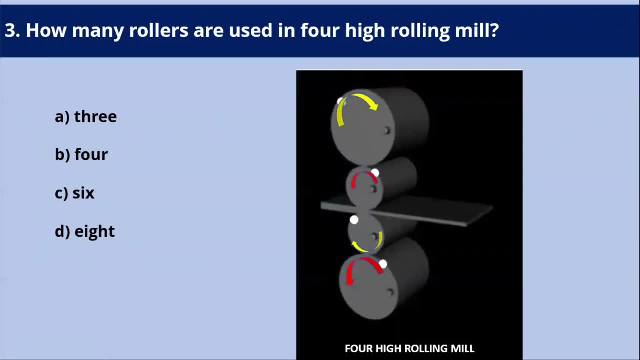 direction of the three rollers. Next question: How many rollers are used in four high rolling mills? So if you see in this diagram, in the four high rolling mills we are using the four rollers which is employed for rolling and the direction of these two rollers is the same and the remaining two. 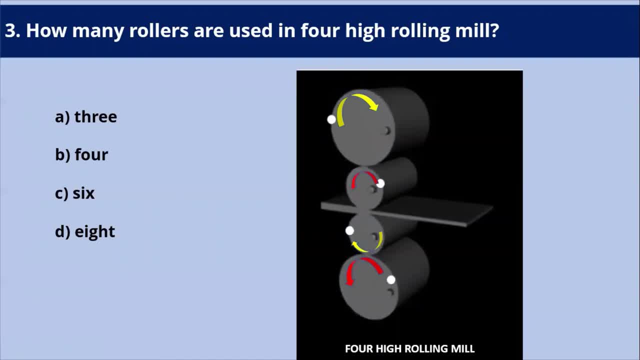 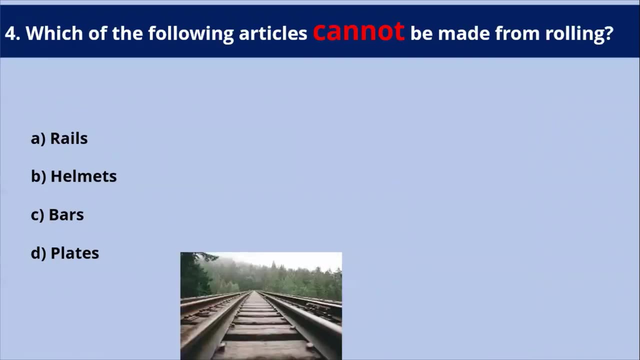 rollers are in the opposite directions. So basically, our answer is four. It means that for a four high rolling mill, we are using the four rollers and we can see the directions for rolling. Ok, Next question: Which of the following articles cannot be made? 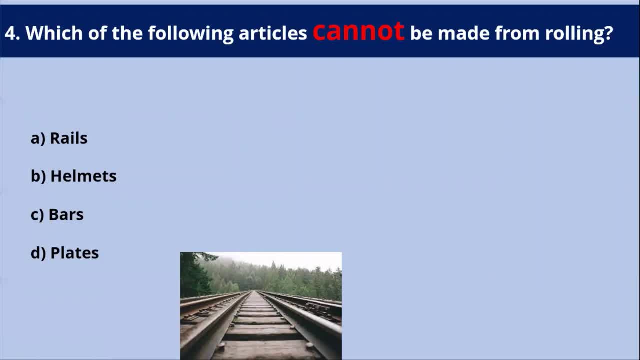 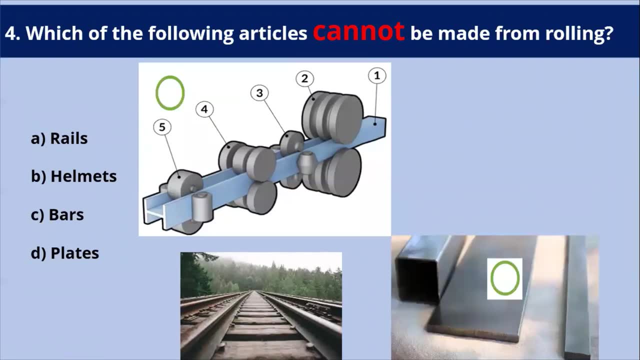 from rolling. No, rolling is a very useful for making the articles, like I can see the rails, or even we can make the bars as well as the plates, But in the rolling mill it is not possible to make helmets. that's why our answer is b, so it means that the in the rolling we can't make the helmets. 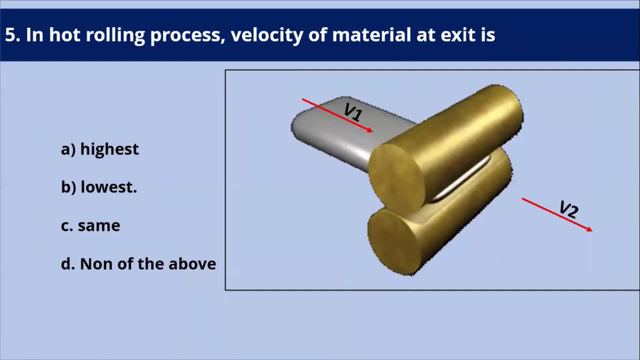 our next question: the in hot rolling process velocity of a material at the exit. exit means this point: v2 is the exit and v1 is the entry point. so the velocity of the workpiece at it when it leaves the roll is greater than the velocity of the material at the entry due to the, i say due to the stretching. 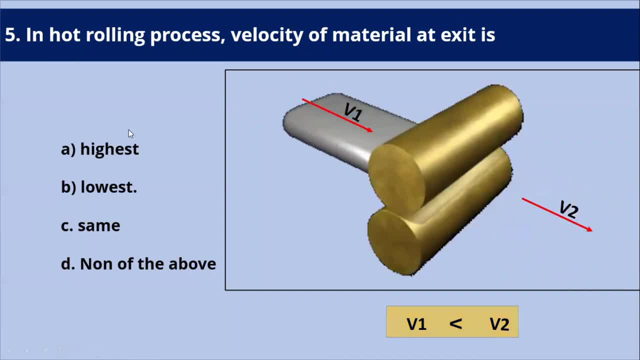 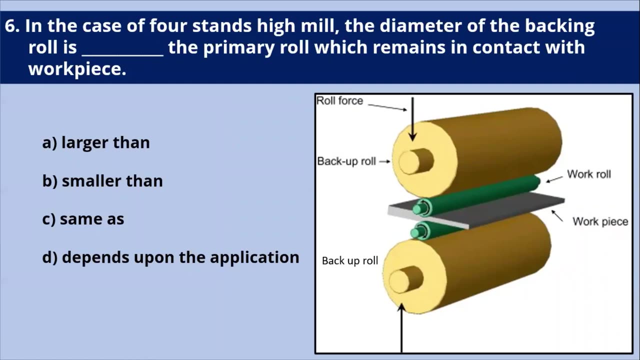 of the layers right, and that's why we can say that the velocity at the exit will be the highest velocity as compared to the, the, the A entry point. next question: in the, in the case of four stand high mill, the diameter of the backing roller roll is dash. 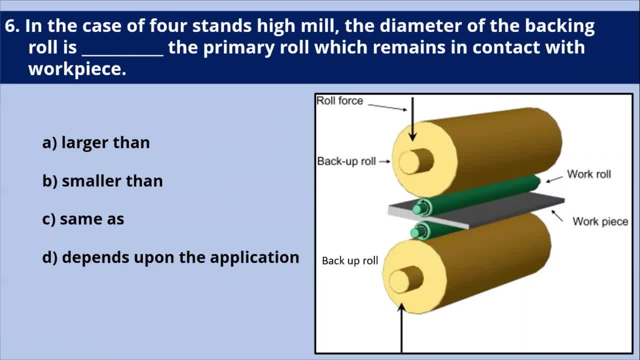 the primary rolls, which remains in contact with the workpiece. now, even in this such cases, the diameter of the you can see the backup roller is diminished, because the diameter is always higher than the working rollers or, I can say, the primary rulers. okay, it. so in such cases, we know that our answer becomes a larger than it means. 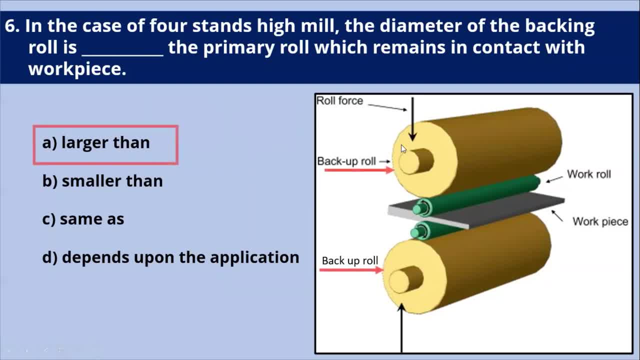 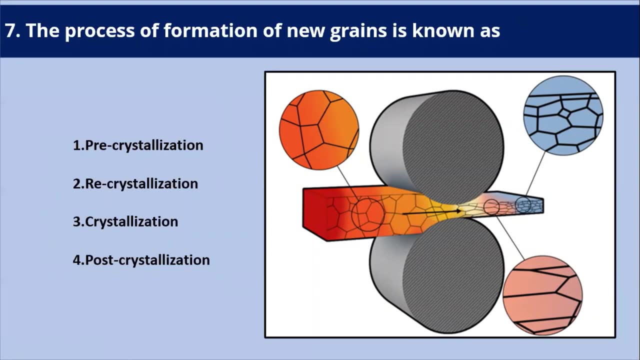 that the diameter of the backing roller is larger than the primary rules, and that's why your answer is a larger than next question is the process of around the roll that the half, and that's why your answer is A larger than next question is: formation of new grains is known as as new grains. when you are generating, it is called as a. 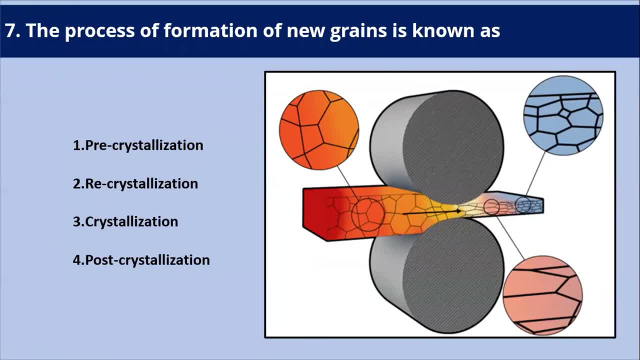 recrystallization: okay, and recrystallization is a process by which the deformed grains are replaced by a new set of defect-free grains- okay, and grow until the original grains have been entirely consumed, and that's why we can say that the the process of formation of new grain. 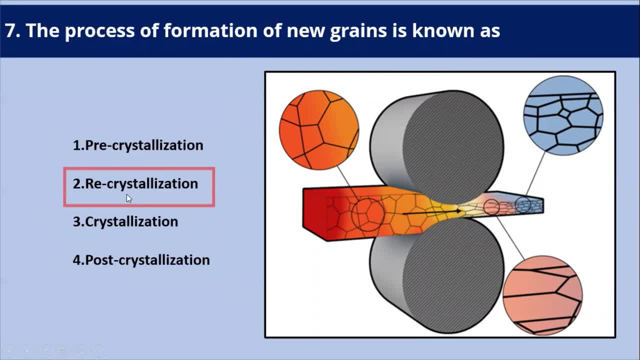 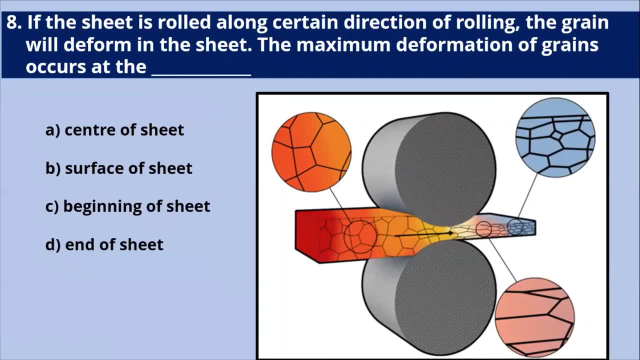 is known as a recrystallization process. okay, next one: if the sheet is rolled along a certain direction of a rolling, the grain will deform. in the sheet the maximum deformation of grains occur at- okay, Now the generally what happens? the grain at the surface of the sheet undergoes the maximum. 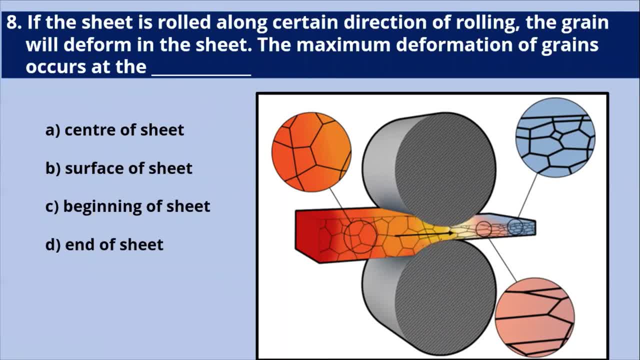 elongation along that rolling direction, while the grain at the center- this is here, so at the center- tends to remain as it is, as it is before the rolling. so that's why we can say that the maximum deformation of the grain occurs at the center surface of the sheet. okay, you can see from this diagram also. next question: 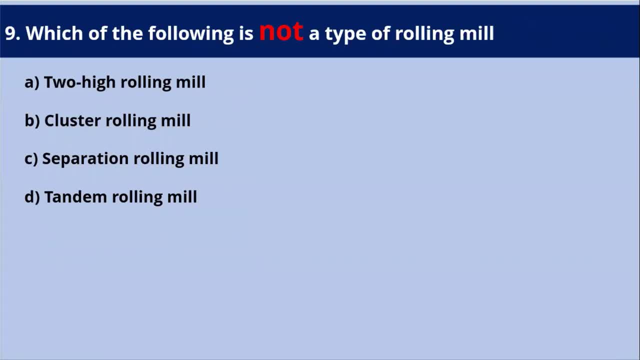 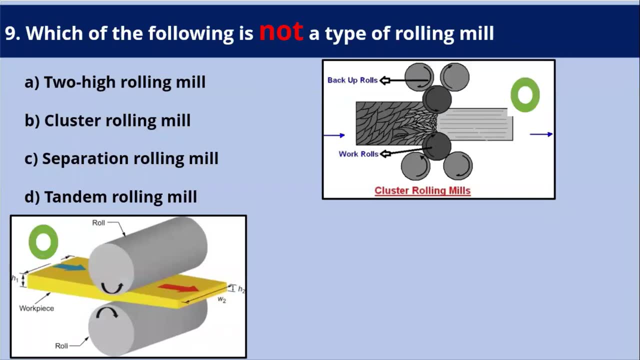 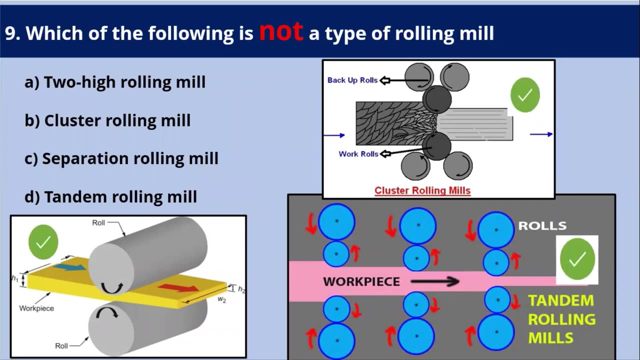 which of the following is not a type of rolling mill? now, i assume that this is a two high rolling mills, this is a cluster rolling mills and tandem rolling mills. all these are the type of rolling mills, but the separation rolling mill is not a type. okay, but in the you know that in two high 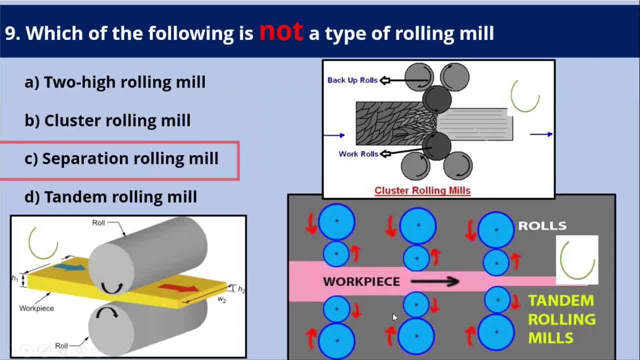 rolling mill. two rollers are rotate in the opposite direction, right and in the cluster we can see here. this is a cluster rolling which consists of two working rollers and four or more backup rolls are there and in this, uh, tendon rolling mills, it is just a special type of 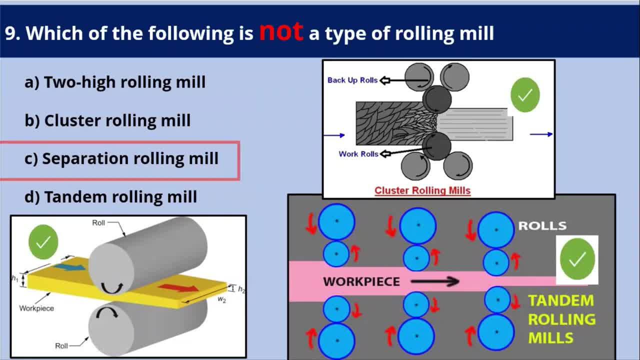 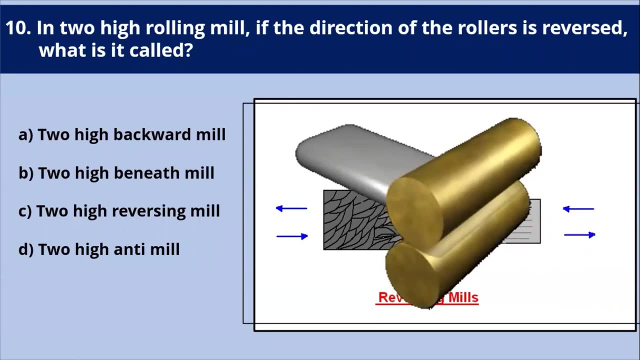 modern rolling mills, mills where rolling is done in one pass or a single pass. so here that's why the separation of rolling is is not a type of a rolling mills. next question: in too high rolling mill, if the direction of the rollers is reverse, so what it is called now from this diagram also, it is very 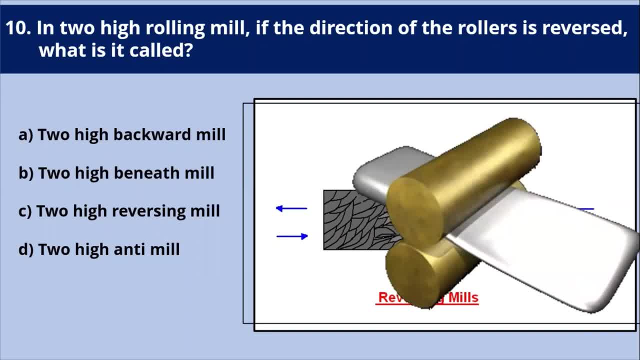 clear that in the too high reversing mill the mill rotate first in a one direction- you can see in the diagram- in the one direction, okay, and then in the other direction means in the other direction, means again the reverse direction right now, so that rolled metal may pass back and forth, means it. 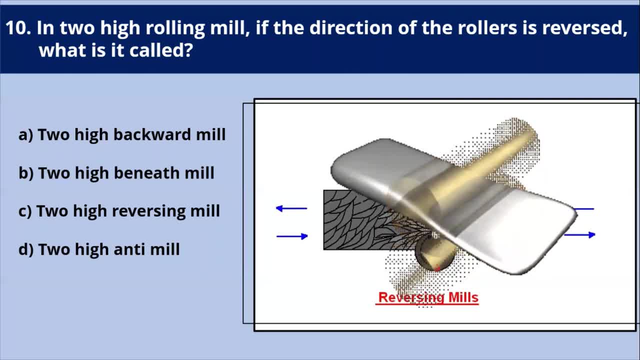 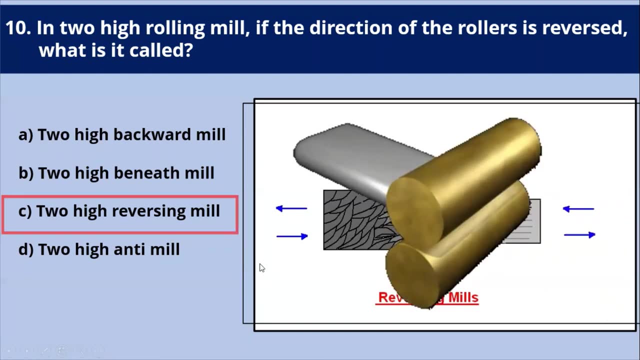 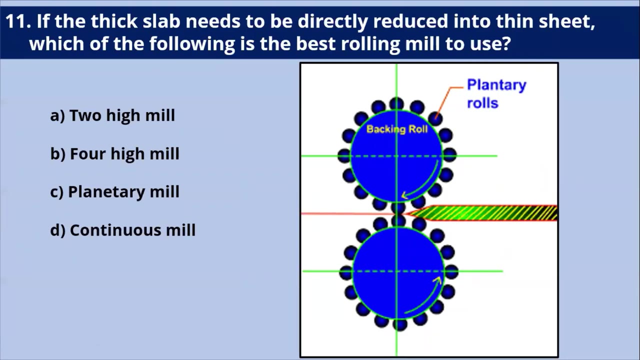 will move forward as well as the backward through the rolls several times, then that system is ultimately called as a rolling mill, as a too high reversing mill. okay, from this diagram i think it is very clear, okay. next question: if the thick slab needs to be directly reduced into thin sheet, which of the 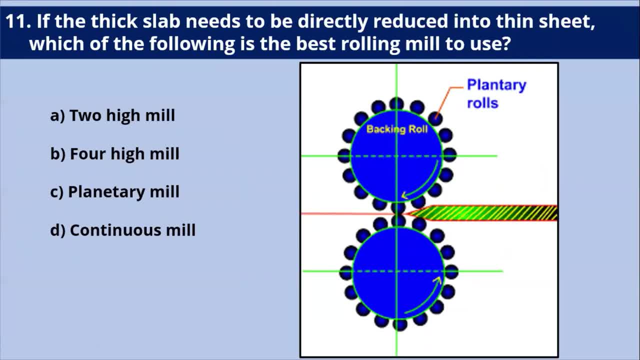 following is the best rolling mill to use. so in this case, too high, or four high, or a continuous rolling mill, so before can't go directly. the reduction of the thin sheet in a um, i can see in the one process, okay, but in the planetary meal, if you see this is a planetary meal, okay, and it is planetary meal. uh, consists of. 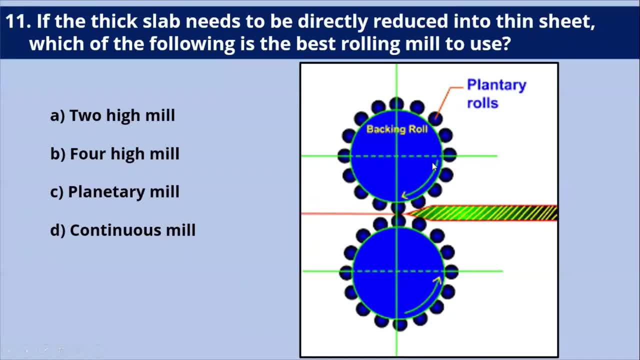 a main role and uh then the backup, with uh supporting roles in a circular arrangements. so the overall reduction is the summation of series of small uh reduction of each pair of roles and therefore we can say that the planetary meal reduced uh directly to the thin sheet in a one pass through the mill and that's why our answer. 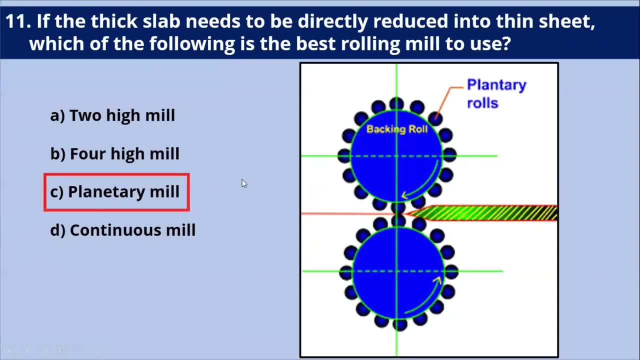 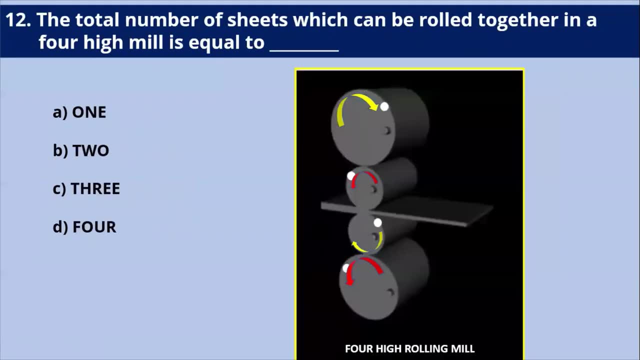 is planetary meal. so you know it's very simple, because in a one pass only the planetary meal is such a rolling type where we can go in a single pass for the reduction, reduction of the thin sheets. next question: the total number of sheets which can be rolled. 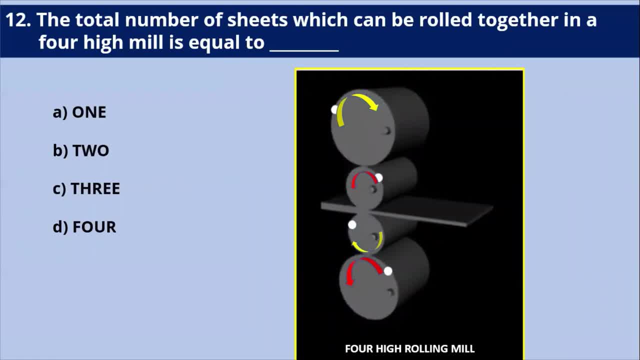 together in a four high mill is equal to. even if you see in this diagram there are four roll bits. okay, but in this four high mill, which consists of a two larger roller and two smaller rollers- okay, that is from the top as well as the bottom and the smaller. 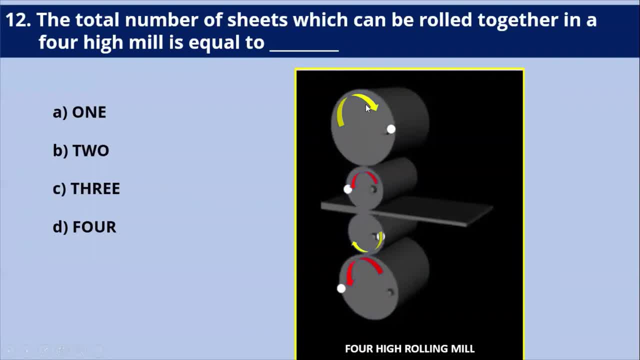 roller is just supported with the help of this larger roller and only a single sheet at a time can be rolled in the in this mill. so whether means basically, they are asking that the in four high rolling mill is equal to how many sheets we can proceed, so only. 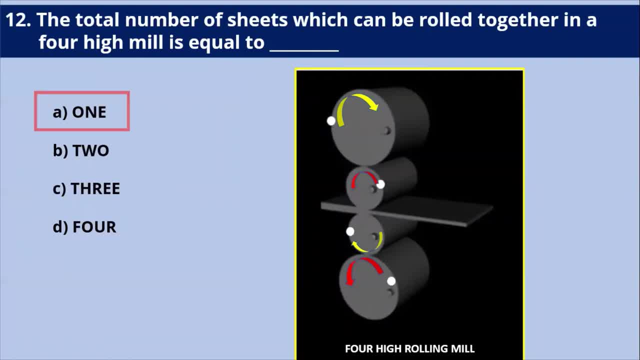 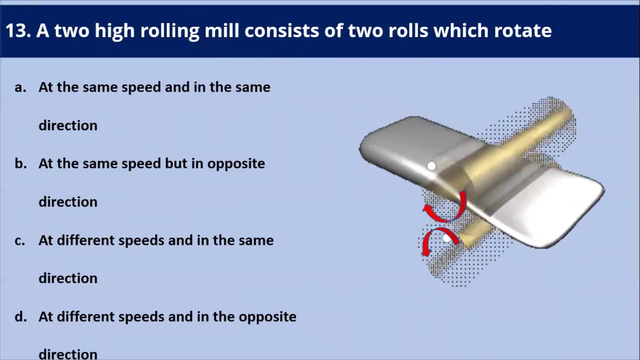 the single sheet. that is a one answer. our next question: a two high rolling mill consists of two rolls which rotate. now from the diagram, if you see the, which one is the correct one? we have to choose here at the same speed and in the same direction. that is the what actually they are talking here. 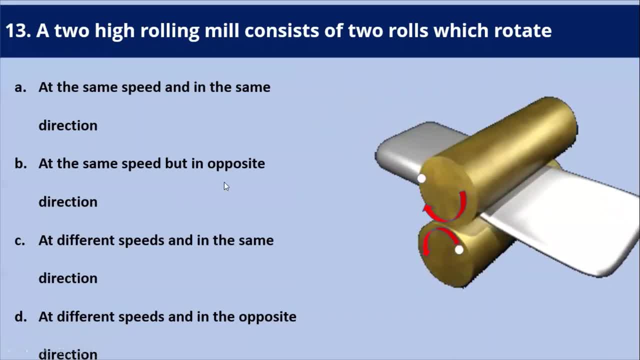 so now, when you do the same thing at the same speed but in the opposite direction, can you see? in this direct direction the speed is same, but in the rollers are rotating in a opposite direction. actually your answer is b. but if you see the other options also at a different speed, no, the speed will always. 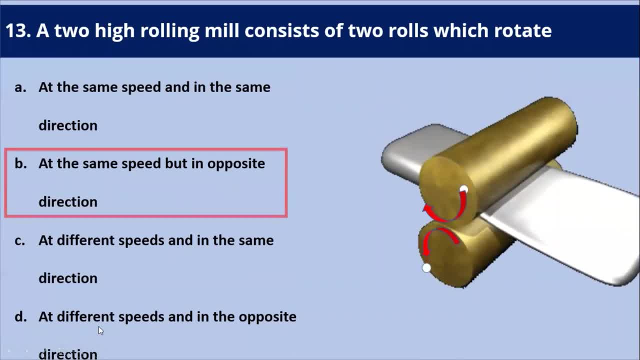 remain the same, even if you go for the fourth option, at a different speed, okay, and in the same direction. even opposite direction is right, but the speed will not be where the opposite direction is, in fact, at an equal distance. now, this is the option which you can use to 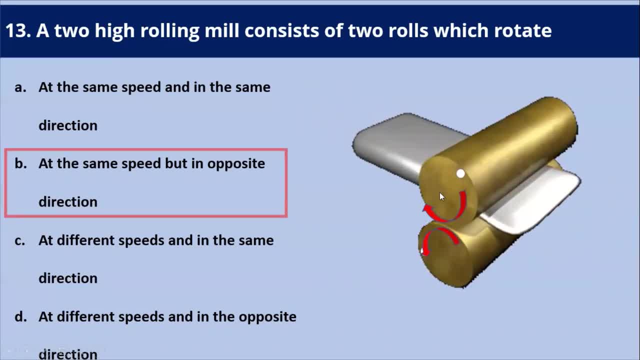 These three things. we have to remember that they do not should be consequences in the other direction. so there is truth in it really mean each value can be taking this everything. so whether you 하igner to say what is the operation if the general direction and vary, okay, here, also at a different speed, he is saying no, the speed will never be a different. 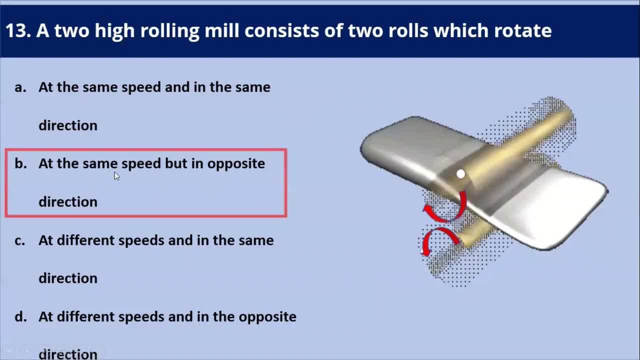 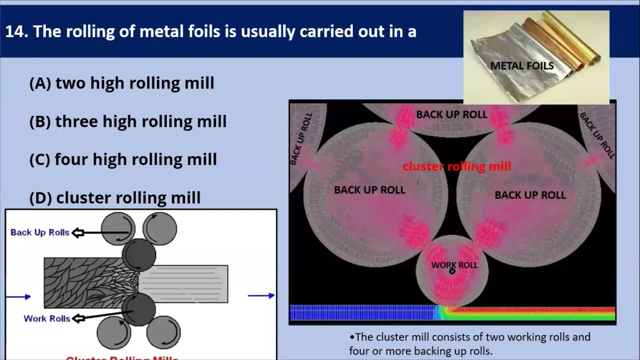 so that's why our answer is that two eye rolling mill consists of a two roller which routed at a same speed but in a opposite direction. next question: the rolling of metal foil is usually carried out in? is usually carried out in a? actually, the answer is the cluster. 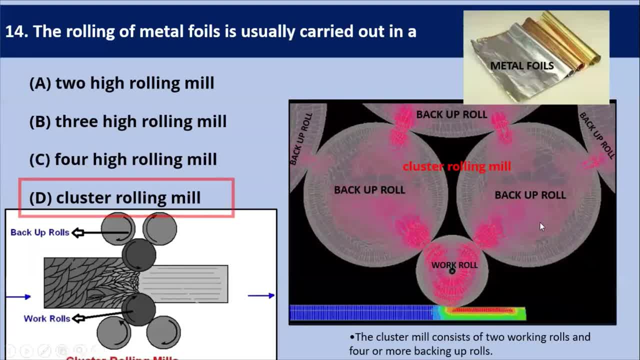 rolling mill. the cluster rolling mill consists of a two working rollers. you can see in this direct: these are the two working rollers, okay, and four, or I can say more than four, backup rollers are there. okay, you can see in this direct, in this diagram, and due to that reasons, 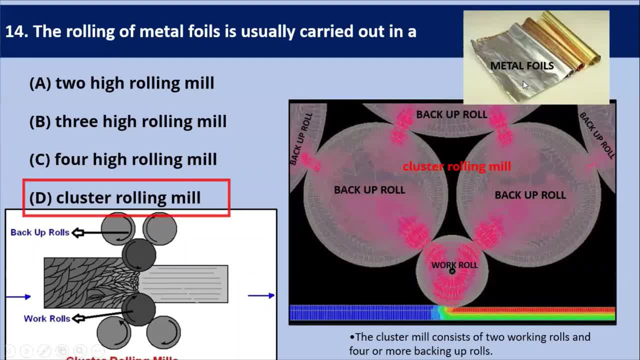 the metal foil Can be. Easily I can say the produce in the cluster rolling mills and the question there in the same way. they are asking the question. no, the rolling of a metal foil is usually carried out, so it is usually carried out in the cluster rolling mills. next question: which of the falling 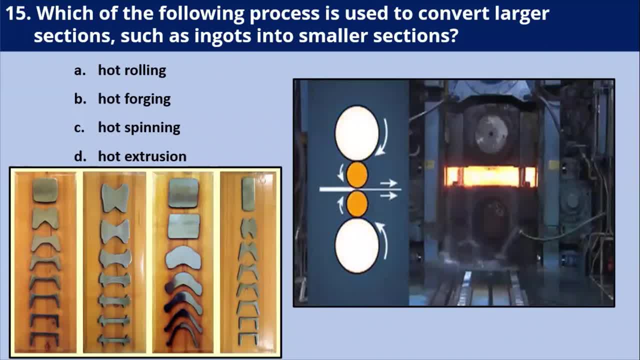 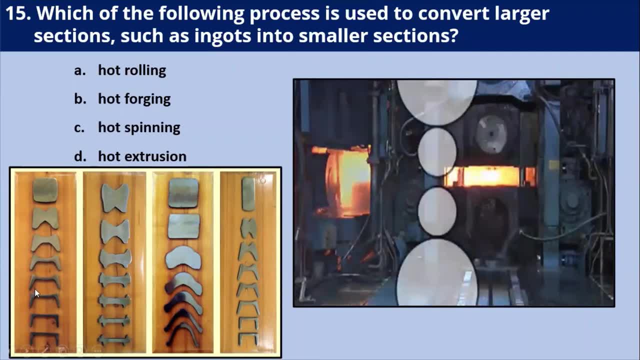 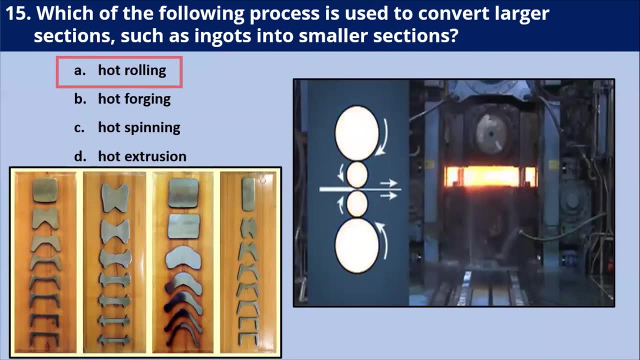 process is used to convert large section- okay, such as ingot, into smaller section means this is a large section And It will be converted into a smaller section so when it is possible- so basically it is possible in the hot rolling- okay, so hot rollers is used to convert the large section into. 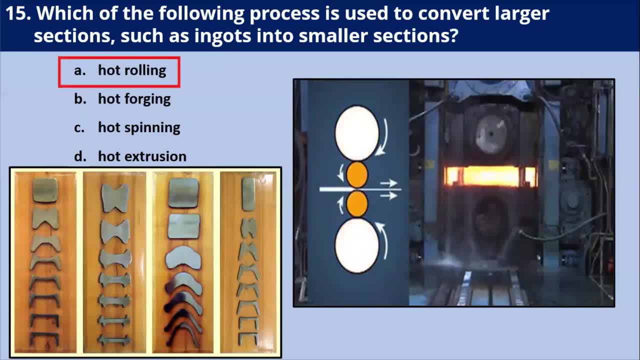 a small section because ingots are heated to a high temperature, around 1100 degree Celsius, and the mill passes the heated ingots through a variable number of stand, which converts the Large section into a small section, and that's why our answer is a hot rolling mill. 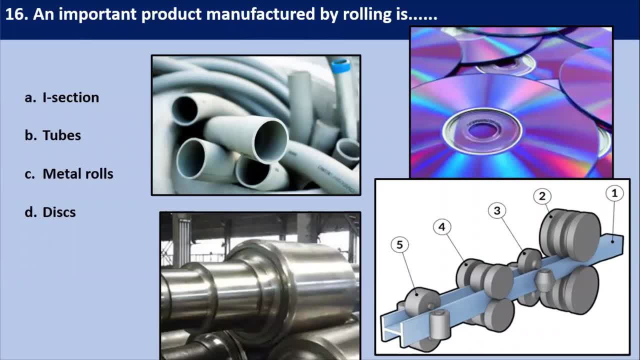 Next question: An important product manufactured by rolling is now, if you see that in the rolling mill we can't produce the tube like parts, even we can't produce the metal rolls also, Even we can't produce the discs, but in the rolling process we can produce the ice section. 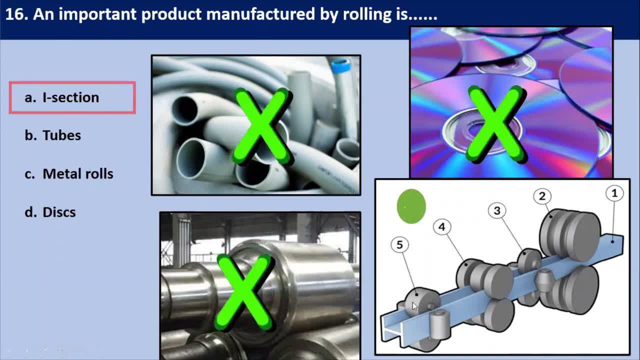 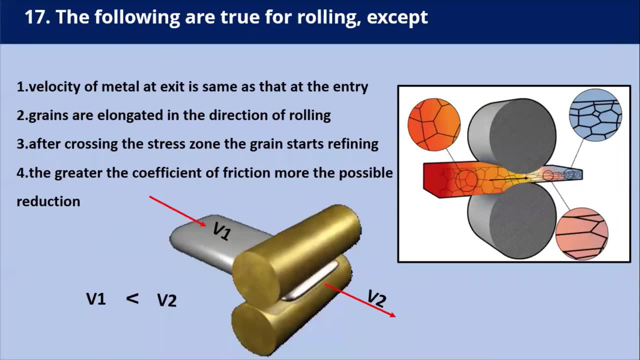 this is called as a ice section beam, and that's why our answer is a ice section. Next question: Which of the following are true for rolling except? okay, now, here also, it's very simple If you see that the velocity of the rolling is very simple. 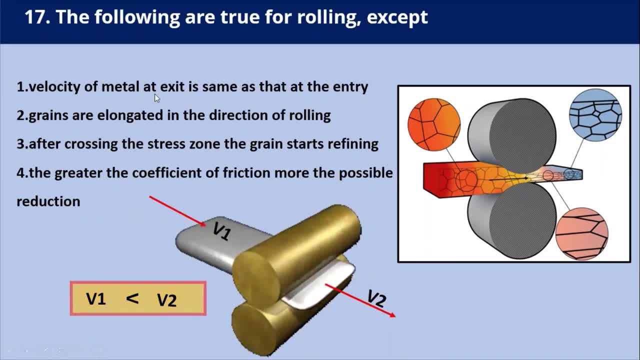 It's very simple. It's very simple. The velocity of the metal at the exit means here at the exit is same as that of the entry. okay means. this is a wrong statement ultimately, even if you see the grains are elongated in the direction of the roll. yes, it is true. okay, even after crossing the stretch zone, the grains 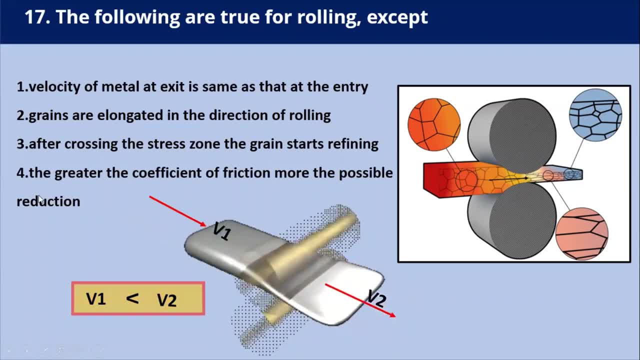 start refining. yes, means this is also true. okay, the greater the coefficient of friction, more the possible reduction. Yes, if there is a more friction between these two will get a more reduction in the ingots, and that's why, in this case, you can say that the answer is velocity of the metal at the 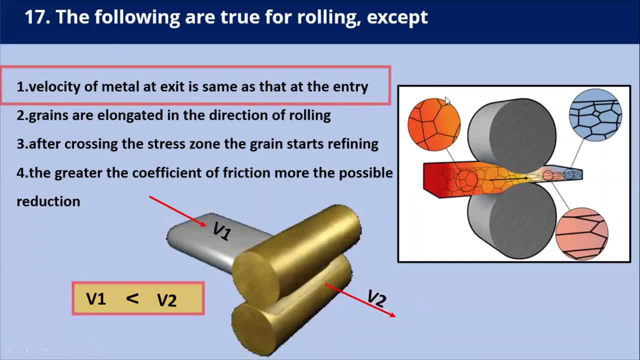 exit is same as that of entry is wrong. okay, we know that the velocities are different at the exit, as well as the at the entry. this is entry and this is the exit, and that's why answer is 1.. Next question: Which of the following are true for rolling except? okay, now here also. it's very simple. 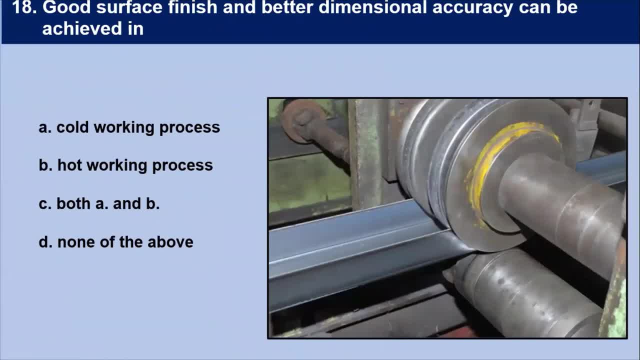 If you see that the velocity of the metal at the exit is same as that of the entry is wrong. then the good surface finish and the good dimensional accuracy can be achieved in. okay, now we know that that hot working process is carried out. about the recrystallization: 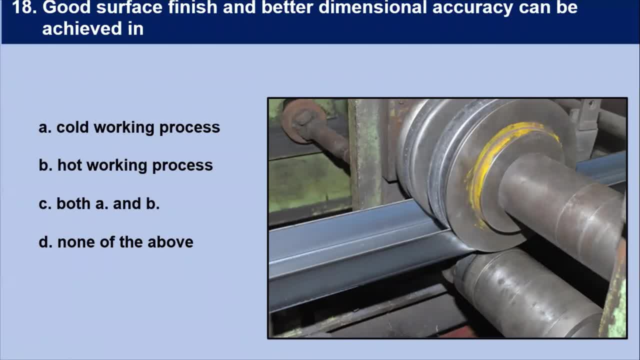 temperature. and after cooling what happened? the metal shrinks slightly and the shape might get changed somewhat there. so we can't achieve the high accuracy. in the hot working process, Okay, but in the cold working process, which is carried out below the recrystallization. 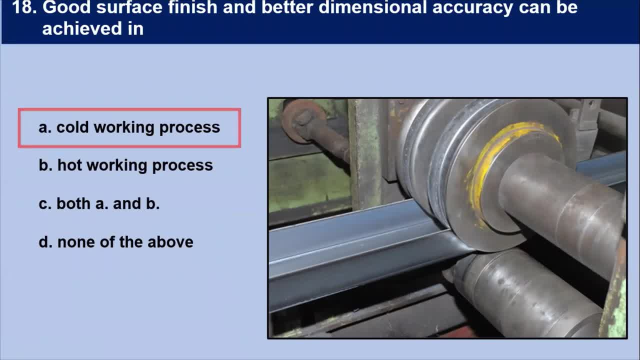 temperature means at the room temperature- which increase the strength and also improve the surface finish and hold a tighter tolerance or a good tolerances. okay, and that's why our answer is: the good surface finish can be achieved or a dimensional accuracy can be achieved in the cold working process. 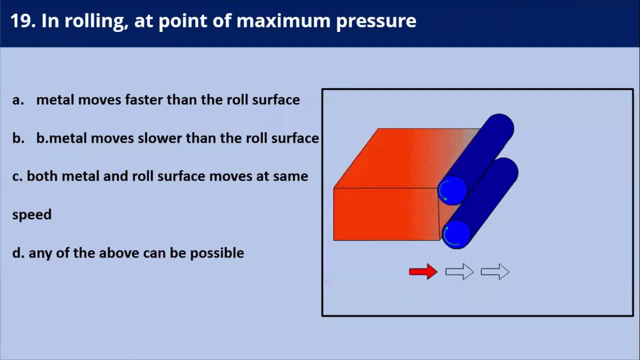 Next question: In rolling at point of maximum pressure? now, what is this question actually? if you see, in this case the? in rolling at the point of maximum pressure means where the maximum pressure exact when both the metals and the roll surface moves at the same speed, means the speed of. 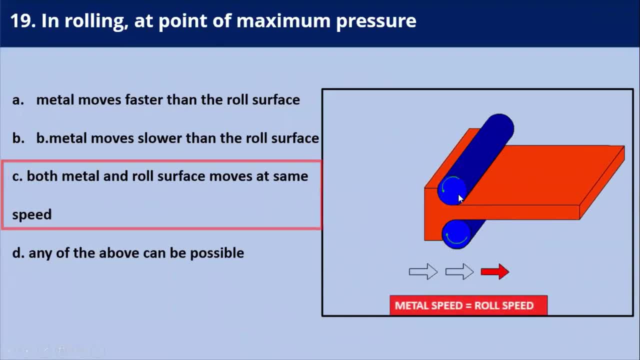 the metal and the speed of this roller. This roller should remain same, than only we can get in a rolling at a max, at a point of maximum pressure. okay, here we'll get a maximum pressure. okay, but the condition is that metal speed should be equal to the rolling speed, and that's why our answer is c. 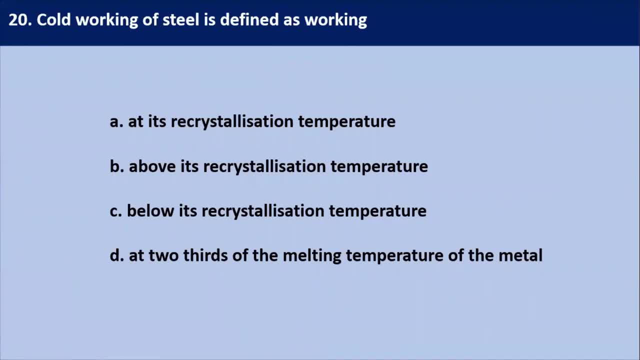 Next question: Cold working of a steel is defined as working. Now, in such cases, We know that. That's why The cold forming, or cold working, is any metal working process in which metal is shaped below its recrystallization temperature, usually at the ambient temperature or the room temperatures. 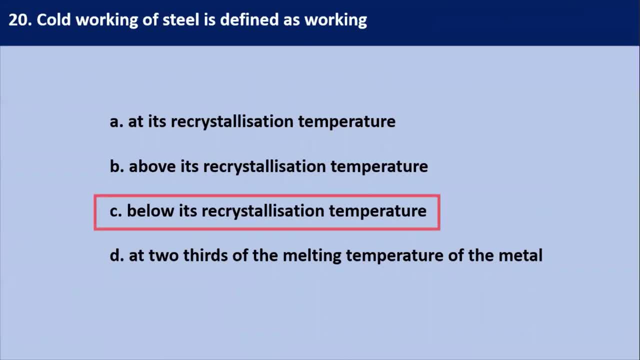 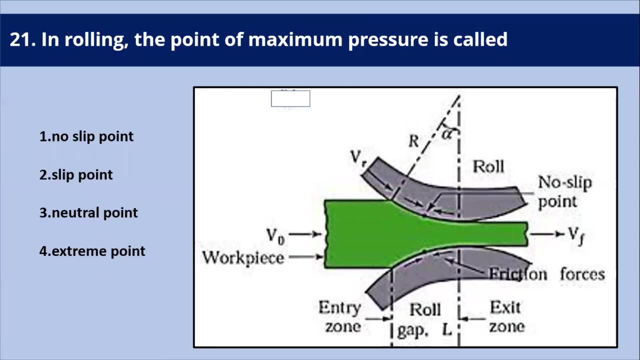 and that's why, in this case, our answer is the below its recrystallization temperature means cold working of a steel is defined as working below the recrystallization temperature. Next question: In rolling, the point of maximum pressure is coils. so what is the name of that point? 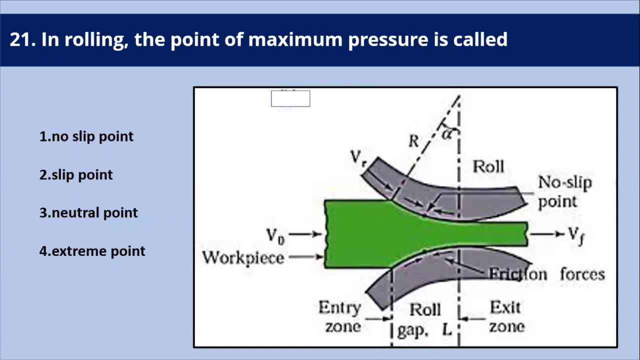 particularly now in rolling process. there is a point on the rolls where the work velocity is equal to the work velocity is equal to the- I can say the roll velocity. okay, so in that case we can see in this diagram at this point, Okay, We will get a no slip point. it means that in rolling the point of maximum pressure is: 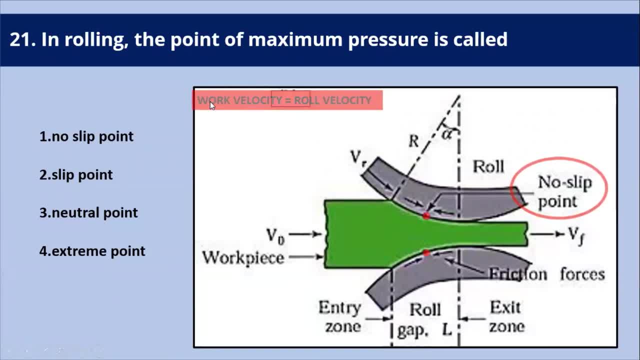 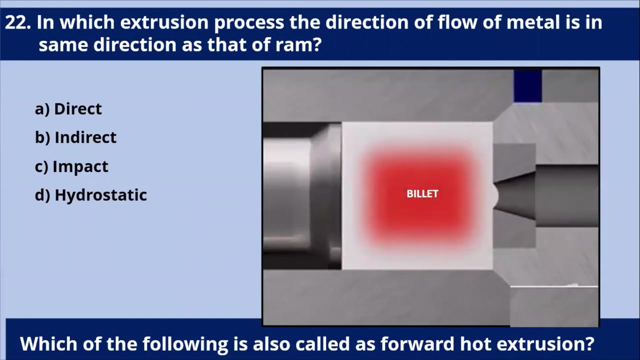 called as a no slip point. but in that case the working velocity- and working velocity is always equal to the roll velocity- and at that case the no slip point can be generated. or you can, we are getting it okay. so that's why our answer is One no slip point. next question: in which extrusion process, the direction of flow of metal? 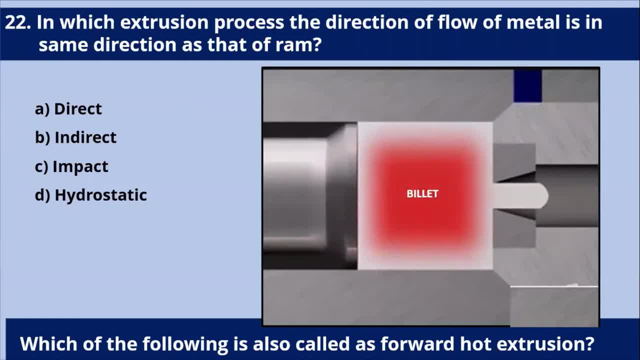 is in same direction as that of ram. actually, this is a question of our extrusion right, even I at the bottom. I read another question also, which of the following is also called as a forward heart extrusion process. Okay, Now we know that in the direct extrusion is a process in which the metal pellet place. 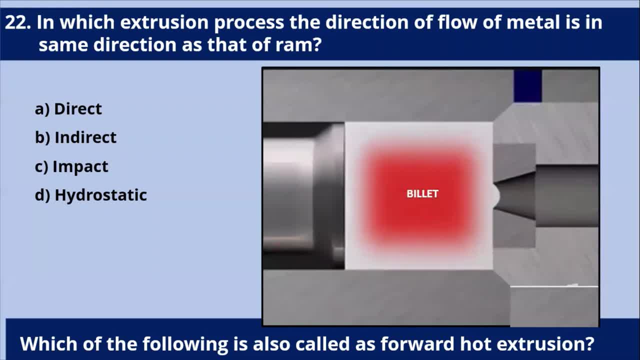 in a container is forced by the ram to pass through this die. you can see, I showed the one die here. okay, and in this type the direction of flow of metal is same as that of direction of the ram. So that's why Your answer is direct. it means that in the direct extrusion process the direction of 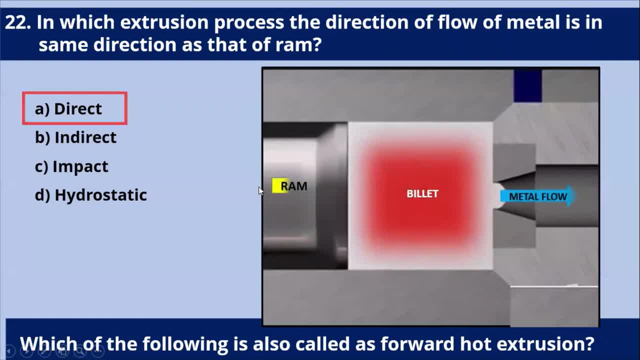 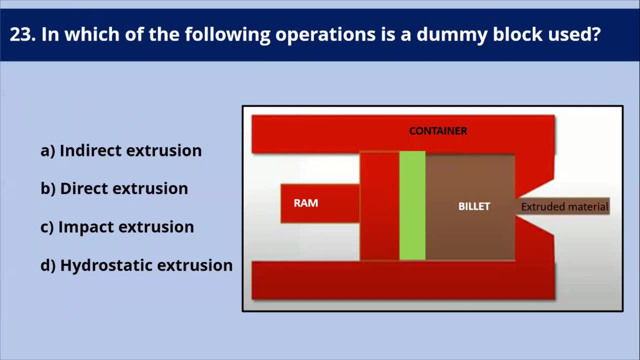 the flow of metal and the flow of, or I can say the direction of the ram is same in the direct extrusion process. Next question: in which of the following operation is a dummy block use? now, this is the what you are showing me diagram. Okay, 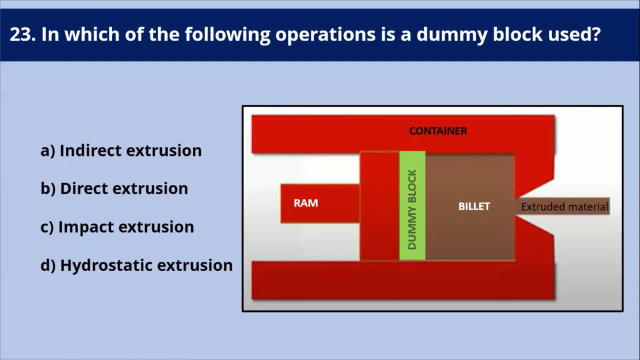 And this diagram. I showed a dummy block right now. basically in a direct extrusion, or I can see the forward extrusion- a dummy block is used during the functioning of this extrusion process to protect the tip of this ram and that's why a dummy block is provided and it means that 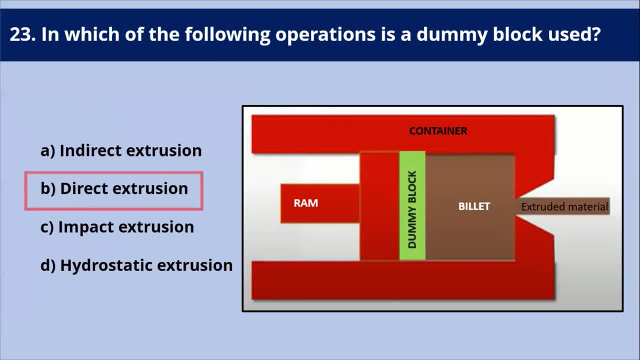 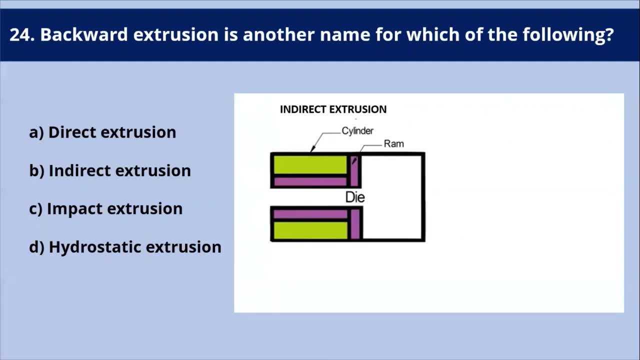 in. In direct extrusion we are using a dummy block. Next question: backward extrusion is an other name for which of the following means: what is the other name of the backward backward extrusion? we know very well that the other name of the backward extrusion is the indirect extrusion. so in this method the metal is extruded. 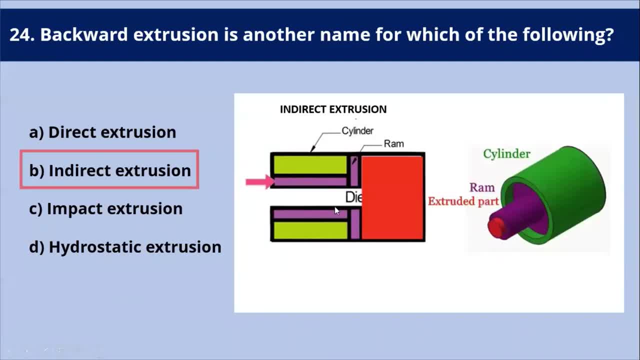 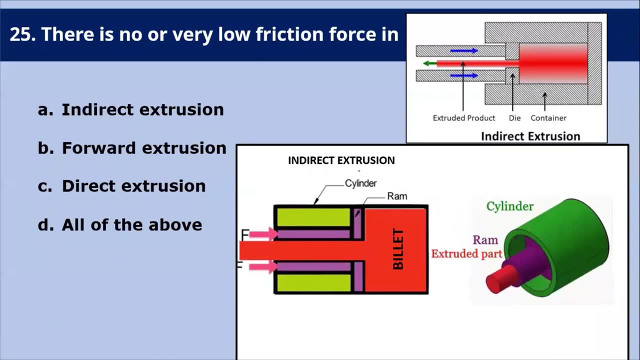 back In the ram or a plunger. you can see from this diagram also. okay, So here the answer is B, indirect extrusion. Next question: there is no or very low friction flow of force in. okay, so the many options they are given and we know that indirect extrusion, or I can say the backward extrusion, does not. 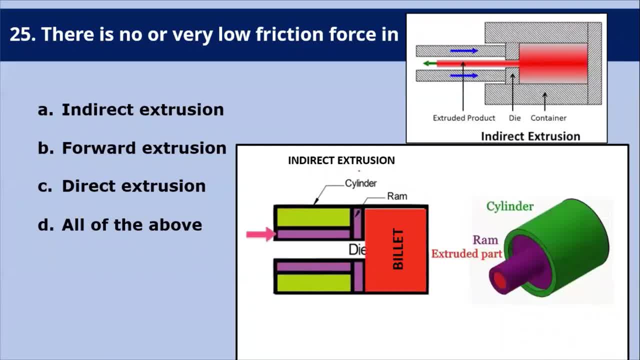 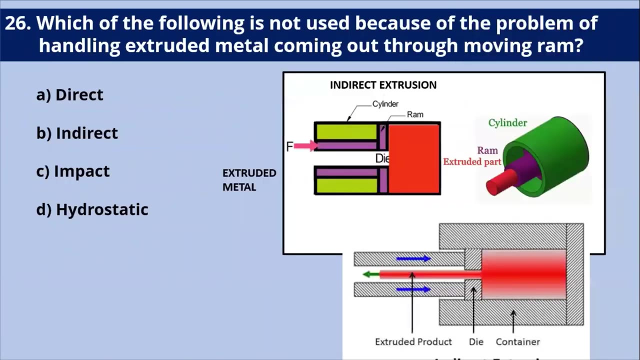 require a large amount of force for operation, as we know that the billet remains stationary. okay, in this, in this diagram also, you can see: the billets remain the stationary in relation to the container and that's why the there will be less friction or a no friction in the indirect extrusion. next, 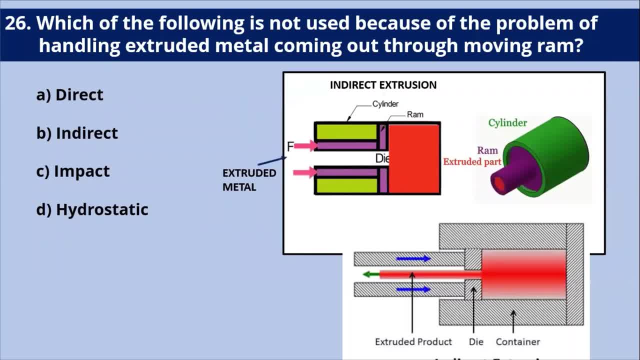 question: which of the following is the indirect extrusion? Next question: which of the following is the indirect extrusion? which of the following is the indirect extrusion is not used because of the problem of handling extruded metal coming out through the moving ram. So when we know that I show the diagram of indirect extrusion or I can say the backward, 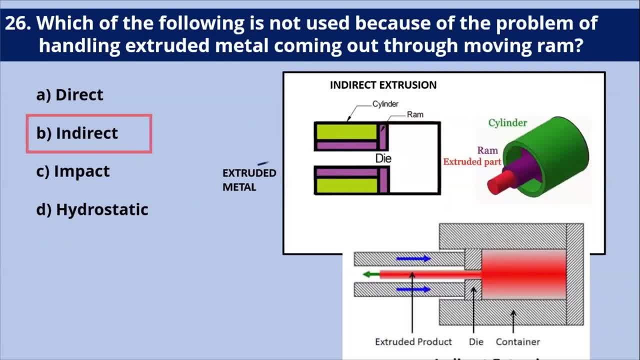 extrusion right. So in this method. basically, why we are not using? because of the problem of handling the extruded metal which is coming out through this moving ram. So you can give a proper support soon, okay, when you get extruded. So here through the die, this die is mounted over the ram. you can see here and then the